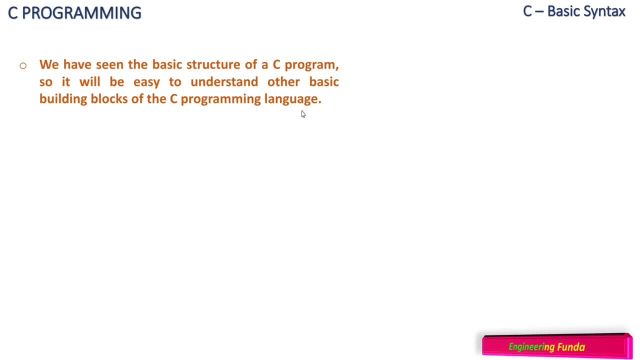 for us to understand the basic building block in a C programming language. so given C program is generally divided into certain basic building blocks and each block is having a specified role in a C program. to get into the detail of that first let us discuss something about tokens in C. now this tokens in C. 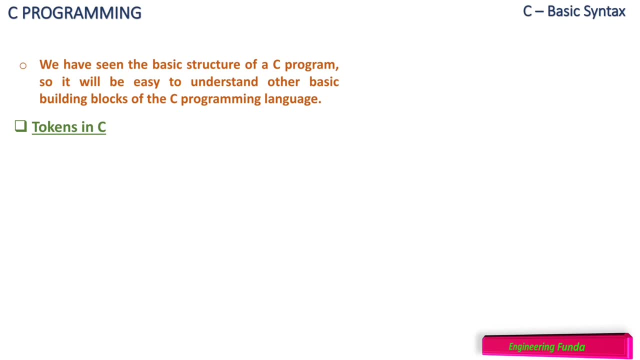 are used by the C compiler to identify whether the given statement is correct or not, it is placed at the correct place or not. a C program consists of various tokens, and a token is either a keyword, an identifier, a constant, a string, literal, or a symbol which has some specified meaning in the C. let us take an example, the following C. 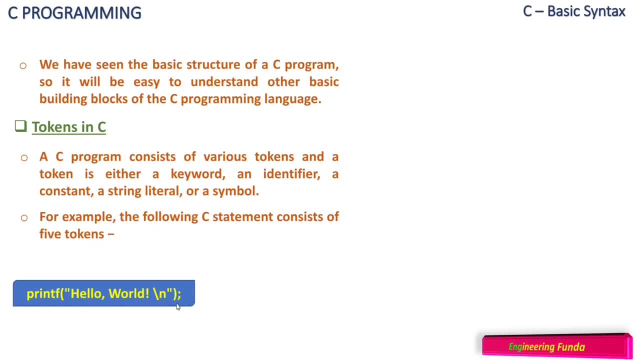 statement consists of five tokens. so the first one is a token and the second one is a token. there is this statement given to us, which is a print statement. printf: hello world, slash n. so there are five tokens in the system. let us see what are those five tokens. 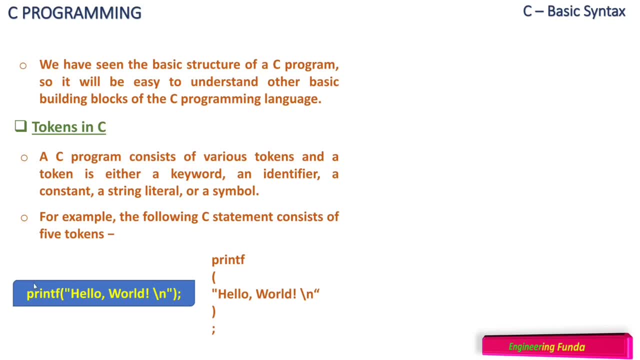 the first token is a printf. this printf, the name of the function which is called to print something onto the screen, is a token. then this opening bracket is a token because this differentiates, this makes the difference between the printf and this string hello world. then this string hello world. from the first letter H to the last character, slash n is a one token in. 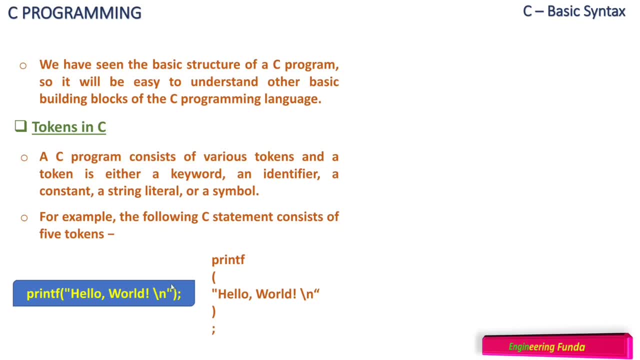 itself, because this is a string and it has to be taken as an whole. then we have this closing bracket as the token identifying the end of the string which is to be printed, and semicolon is the token which is a terminating character for this statement or any statement in a C Program. 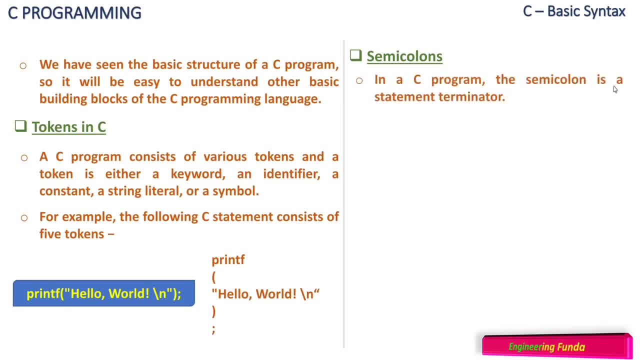 semi-colons. in a C program, the semicolon is a statement Terminator, so every statement is terminated by a semicolon. that is, each individual statement must be ended with the semicolon, Because the compiler understands that the end of the statement is with this semicolon. 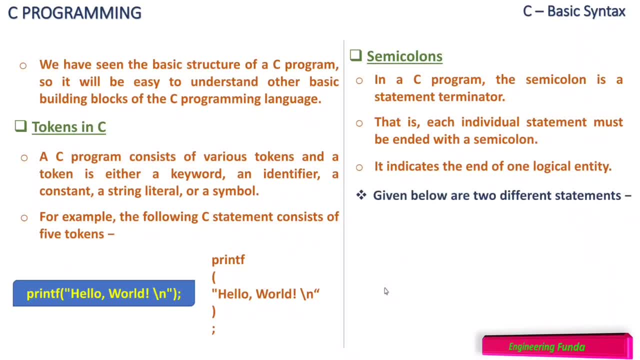 It indicates the end of one logical entity. So given below are the two different statements: printf: hello world, slash n and this semicolon and return zero. So this two statements are ended up with semicolon and the compiler will understand that this is one statement and this is another statement. 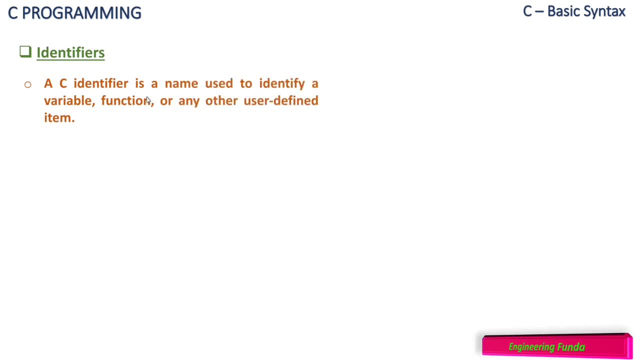 Identifiers. a C identifier is a name used to identify a variable, a function or any other user defined item. Because in a C program We can declare a variable, We can define our own function, or even there are built in functions and we can have some. 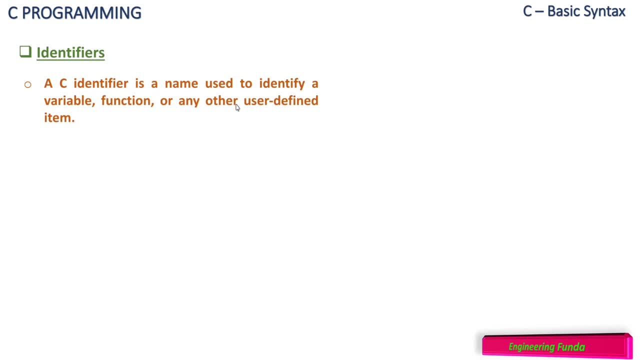 user defined items that we will see later. All of these are identified by an identifier. An identifier starts with a letter- A to Z, capital A to Z or small a to Z or an underscore, followed by zero or more Letters, underscores and digits. 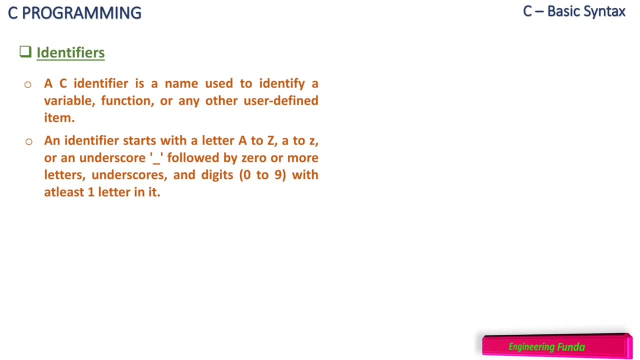 So it should start with A to Z, either in capital or in small letters, And it can also start with an underscore, followed by zero or more letters, underscores and digits, with at least one letter in it. So if it is starting with underscore, then it should have at least one letter. 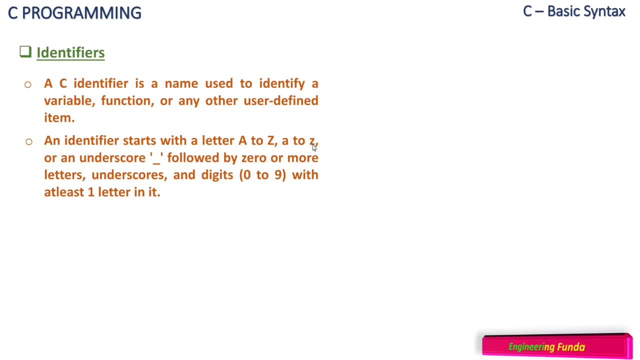 But if it is starting with a letter, then a single letter can be used as an identifier, But a single digit or digit followed by underscore or underscore followed by a digit cannot be used as an identifier. It should have at least one letter in it. 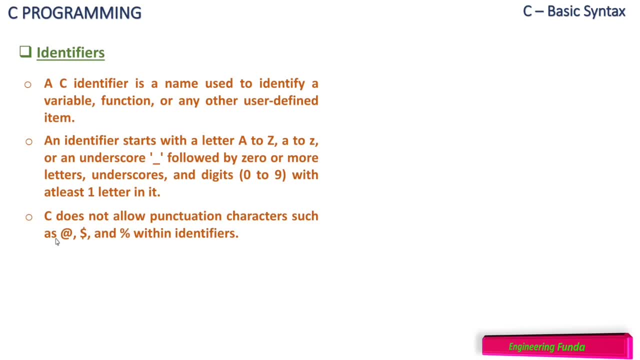 C does not allow punctuation characters such as at the rate, dollar and ampersand within an identifier. The only character, Only punctuation mark that is allowed is underscored. C is a case sensitive programming language. That means the word manpower with an M capital and all the letters small and manpower with 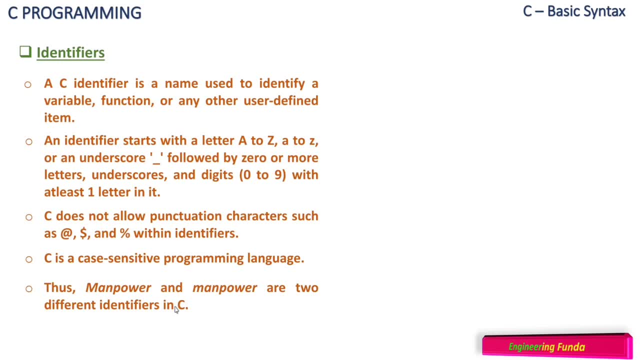 all the letters small are two different identifiers in C, So capital M and small M differentiates the two words And same way if you change any letter either to capital or to small, then it becomes a different identifier. Here are some examples of acceptable identifiers: 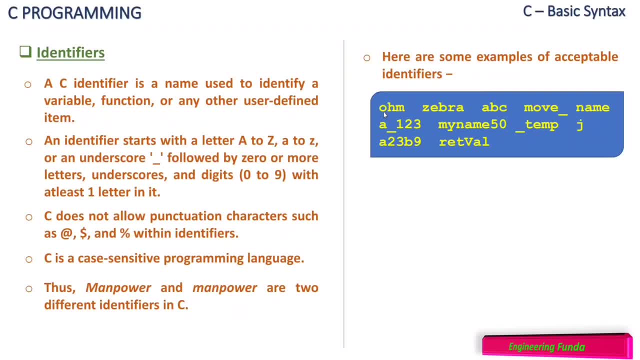 OHM, OM. all letters are identifiers. Zebra is an identifier, ABC is an identifier. Moog underscore is an identifier And this is an identifier. Name is an identifier. A underscore 123 is a valid identifier. My name 50 is valid identifier. 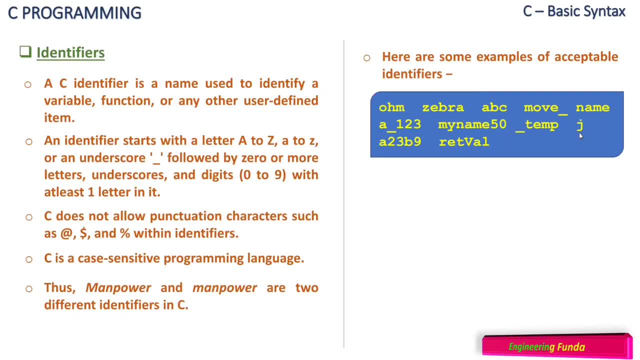 Underscore temp is okay And single letter J is a valid identifier. Then A23B9 is a valid identifier. Same way red well, where V is capital, other all letters are small- is a valid identifier. So these are some acceptable identifiers in C program. 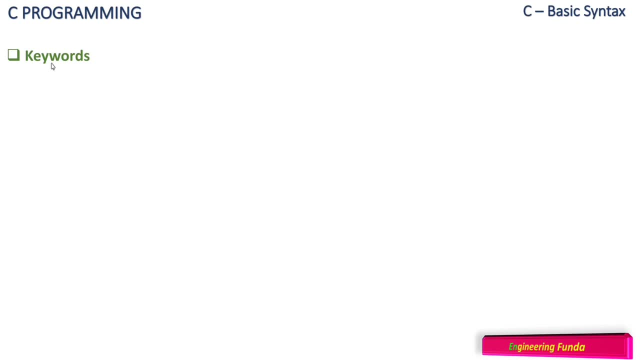 Then there are certain keywords in C program. Now, what is a keyword? Let us look at the definition. These reserved words cannot be used as a constant or variable or any other identifier name. So there are certain keywords in C which we cannot use as an identifier name for a variable. 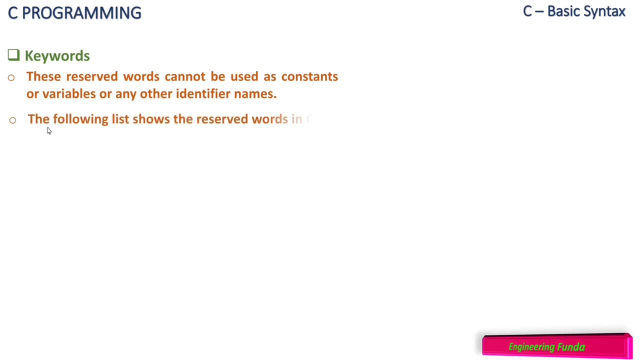 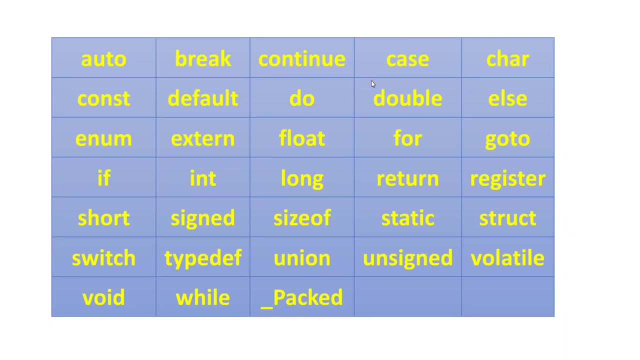 or for a function name, The following list. So It shows the reserved words in a C program. So here this is a table which contains the list of identifiers which are a keyword in a C program. This you cannot use as a variable or an user defined identifier. 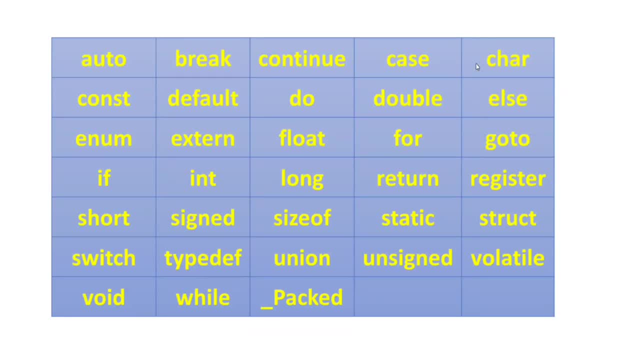 Auto AUTO break, continue case care cons default do, and there is a big list Here. You can see that Useizeoftypedepwhileif. These are all identifier and you cannot have them as a variable name. 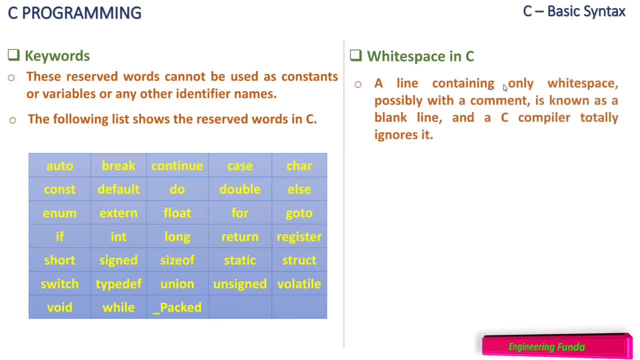 White space. in C, A line containing only white space, possibly with a comment, is known as a blank line and the C compiler totally ignores it. because the C compiler ignores all the comment line and only comment line can have additional or access number of whitespaces. 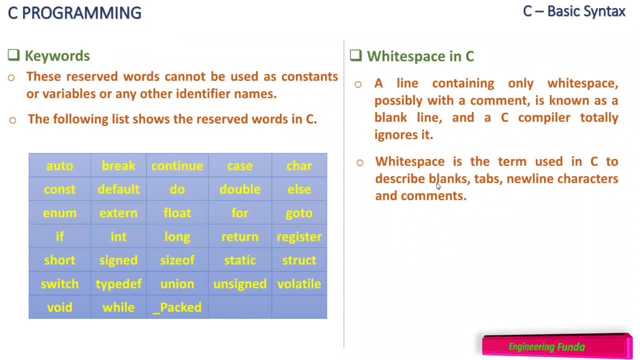 Whitespace in terms used in C to describe blank tab, newline characters or comments. Whitespace separates one part of the statement from another and enables the compiler to identify where one element in the statement ends and the next element begins. So whitespaces are very important. 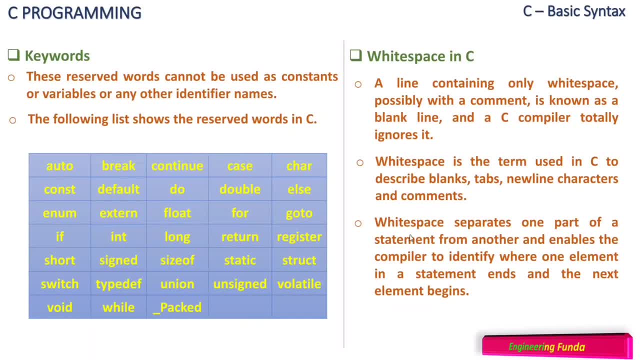 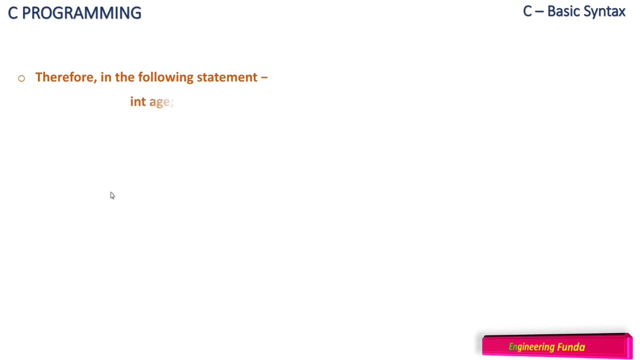 These are used to separate the two entities in a one single statement. Therefore, in the following statement, int age, where there is a whitespace between int and age, separates the int and the age. There must be at least one whitespace character between int and age for the compiler to able. 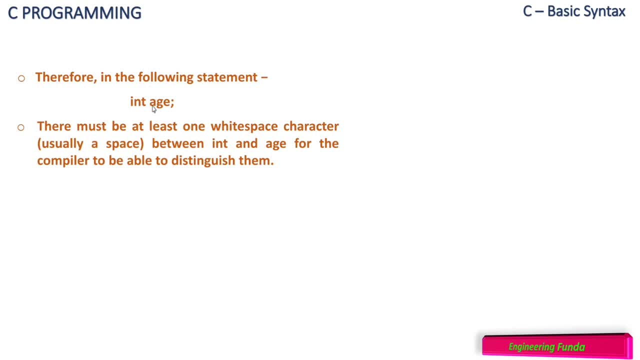 to distinguish them, because if there is no whitespace, the compiler will not be able to understand where the first word ends and where the second word begins. So if there is this one whitespace, there should be at least one whitespace. Then it can understand that this int, where int is a keyword used for declaring an integer. 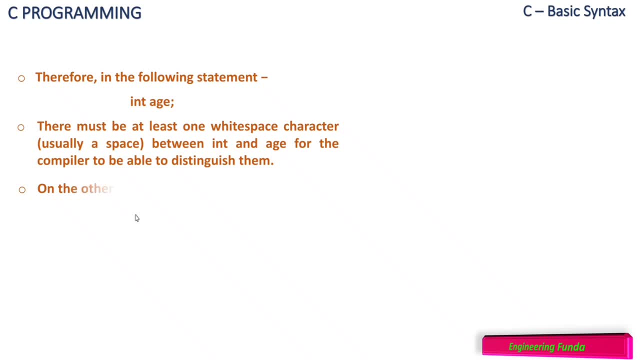 and age is a variable name or the identifier name. On the other hand, in the following statement- so there is this statement, fruit- then there is whitespace equal to space apples plus space plus space oranges. that gets the total number of fruits. So apples, number of apples plus number of oranges will give us number of fruits.